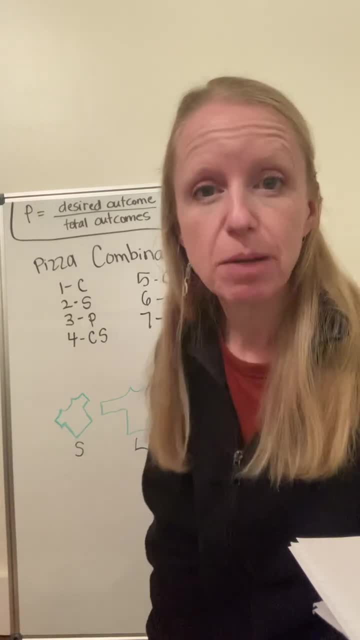 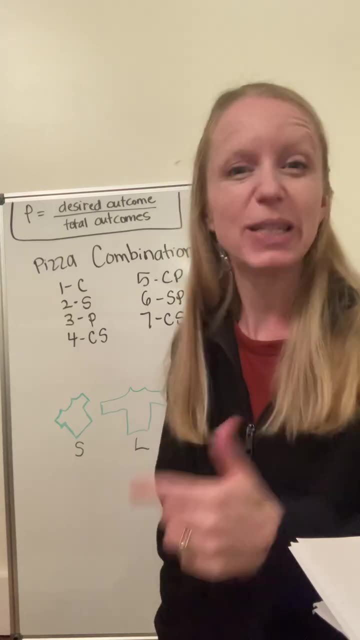 estimation of a large group, And so today we're talking about combination. So this idea of sampling or combination or other things we're going to- permutations we'll mention today, or other things we're going to talk about later on- are just 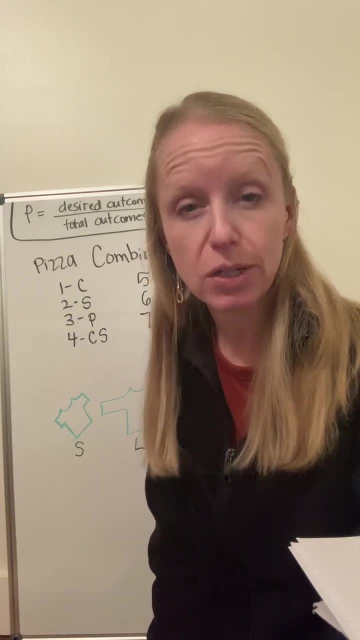 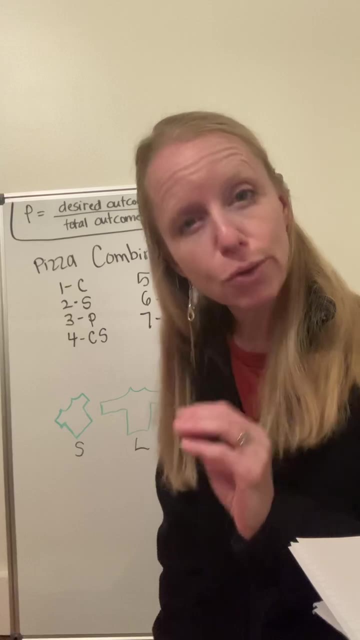 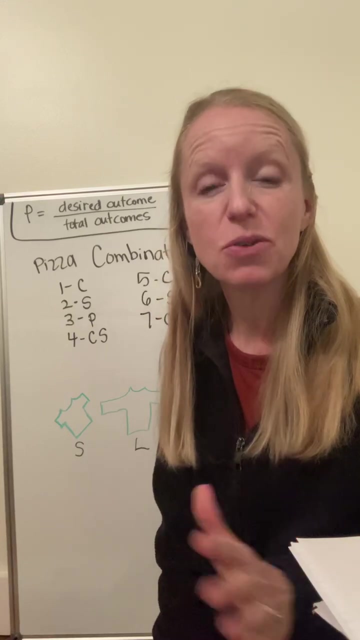 different probability dilemmas or questions. So we had talked about the first week that everything besides God has a certain percentage of chance And so with everything in this world has a percentage of chance, there's all kinds of dilemmas and probability questions out there. 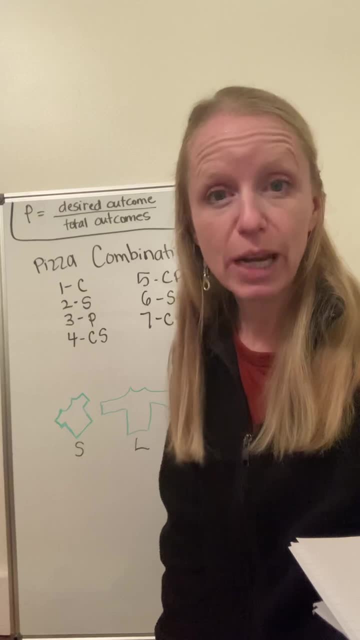 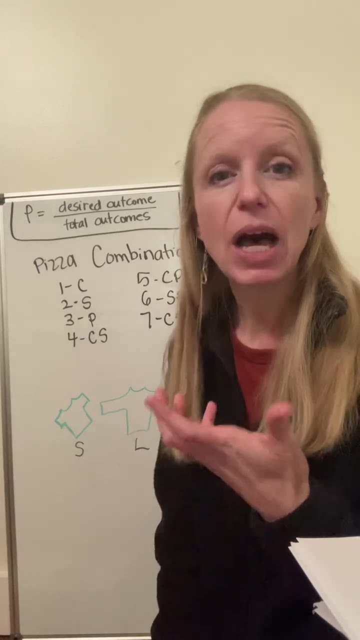 And so we're just kind of again learning the grammar of the different kind of probability dilemmas, And so that's what the sampling was, that is, what combination is It's just looking at a different kind of probability concern dilemma? 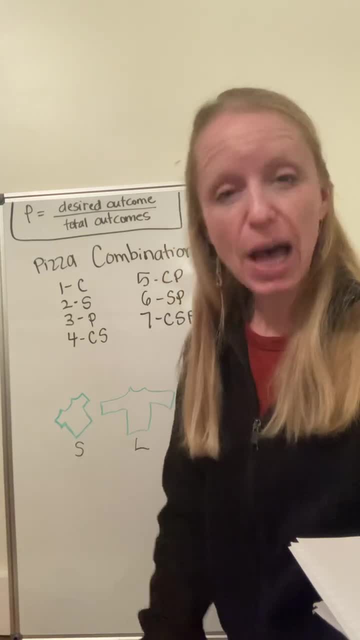 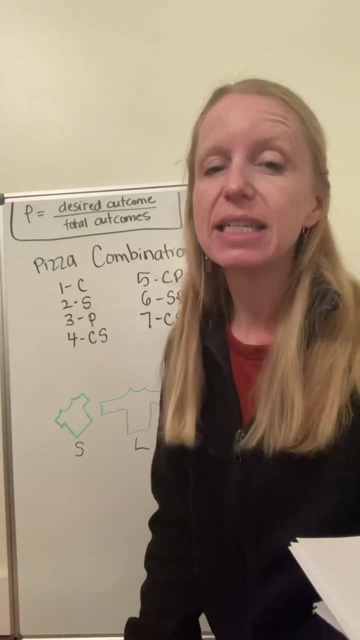 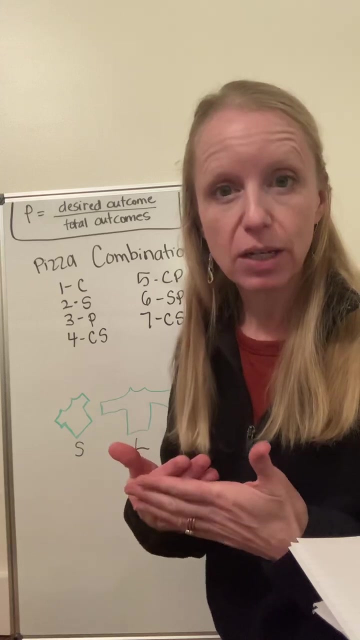 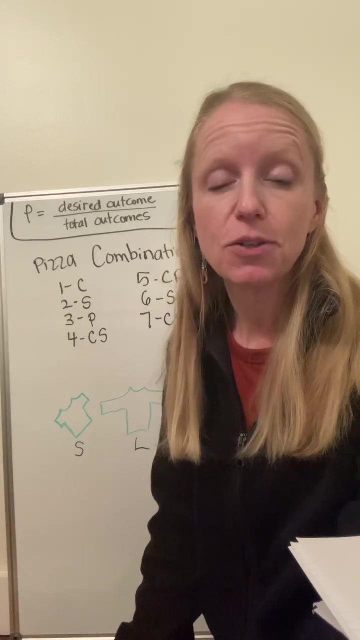 question, whatever you want to call it. and so combination is an arrangement of objects in which the order does not matter, So the order of how you combine the subjects in your question do not matter, And that is what a combination combination is called, or that's the definition of a combination. so today, 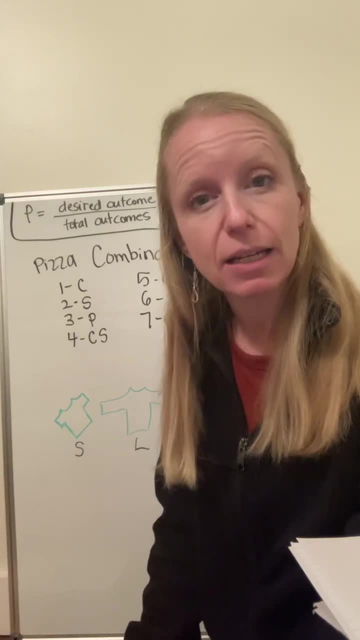 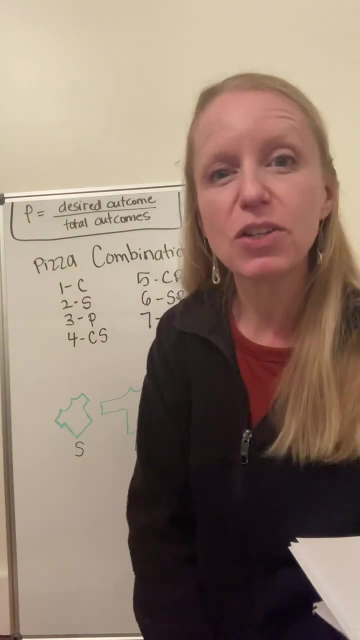 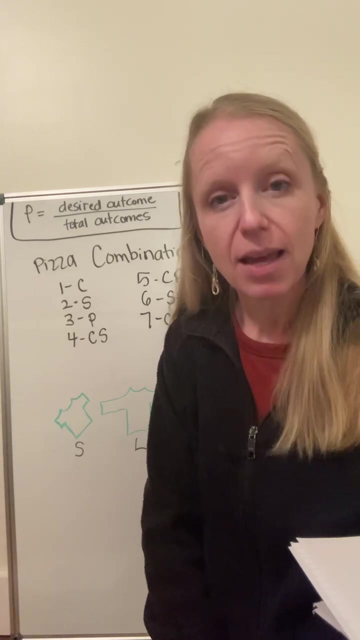 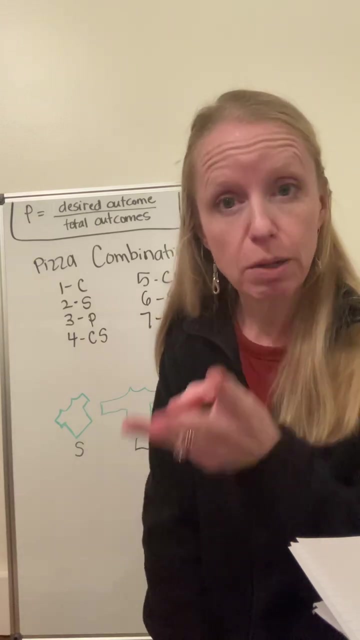 we're gonna look at a combination- probability, concern or dilemma, like the word dilemma- and so the guide gives us the question of entering a pizza place, and so you're gonna ask your kids if you were to walk into a pizza place and they only have three ingredients: they have cheese, they have pepperoni and they have 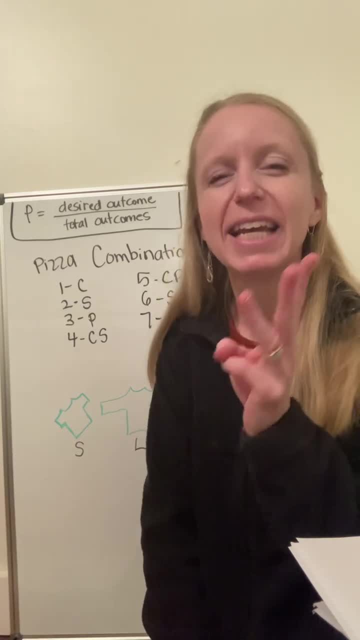 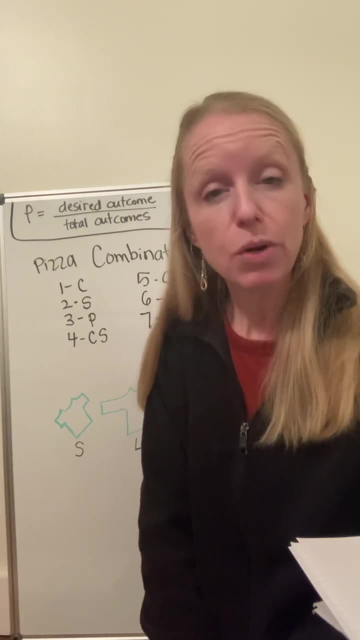 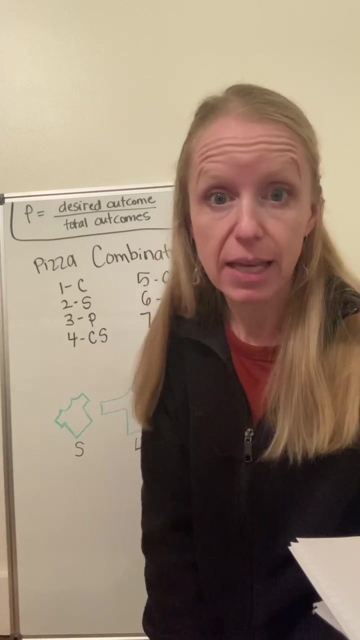 red and red pepper- excuse me, red peppers- what is the probability that you're gonna get the pizza that you want, and what do we have to figure out to know that? well, we have to know, using those three ingredients, what are all the different kinds of pizzas they can make, and then we decide which one we want. and 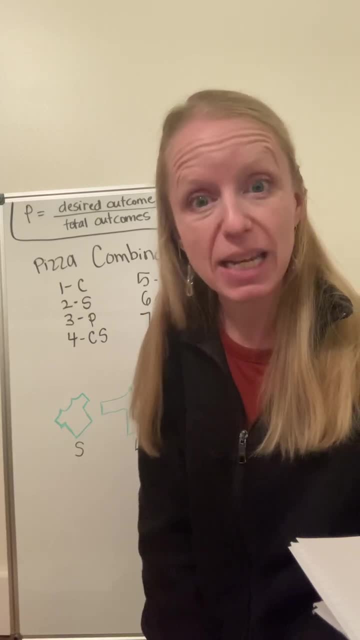 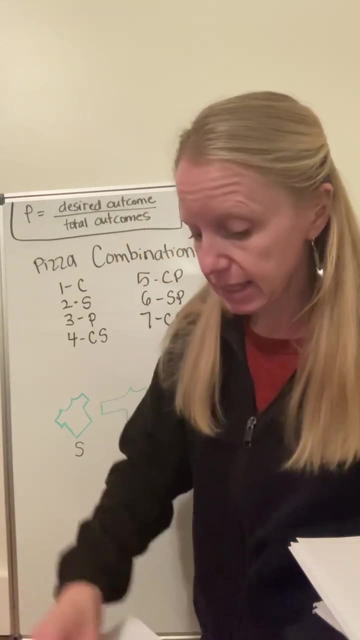 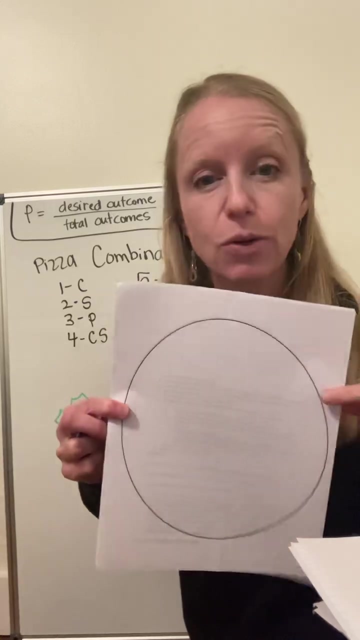 then we'd figure out the probability that we would get the combination or arrangement of ingredients that we would desire. so and I'm going to show you how to do that. So in our classes, each kid will get their get a cardstock with a big pizza circle on it. 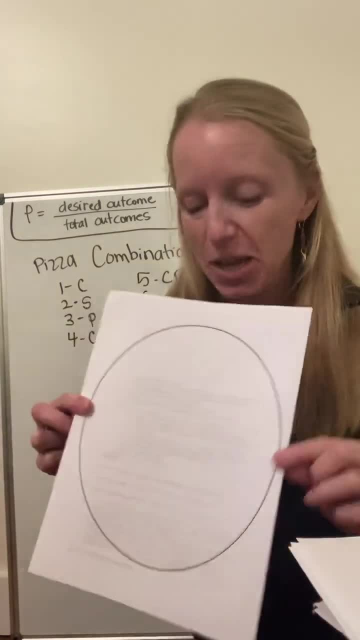 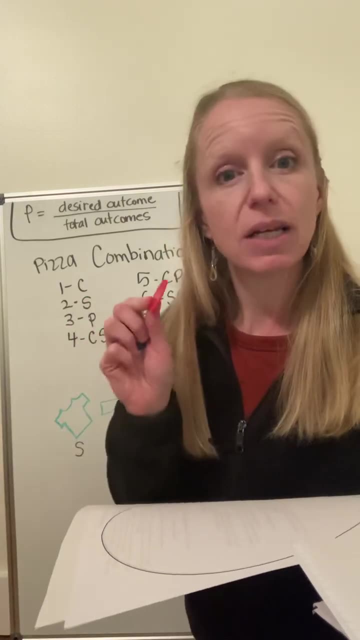 they won't have the words behind it like this one does, but so they'll have their own pizza. and then you're gonna give each student a red chip that's going to symbolize red peppers, the blue chip that's going to symbolize pepperoni, or 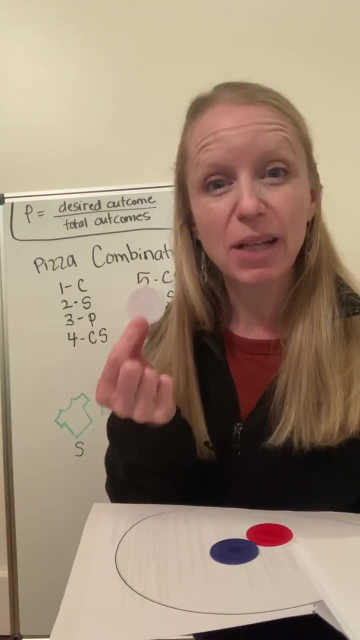 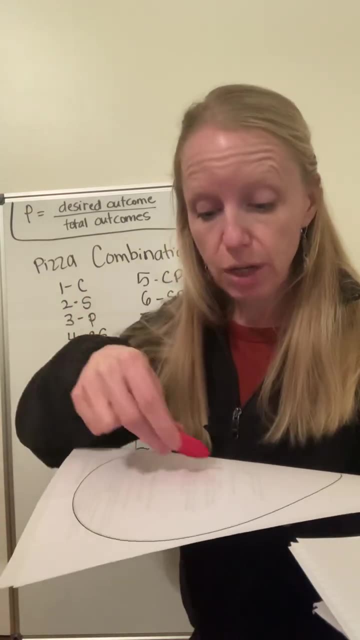 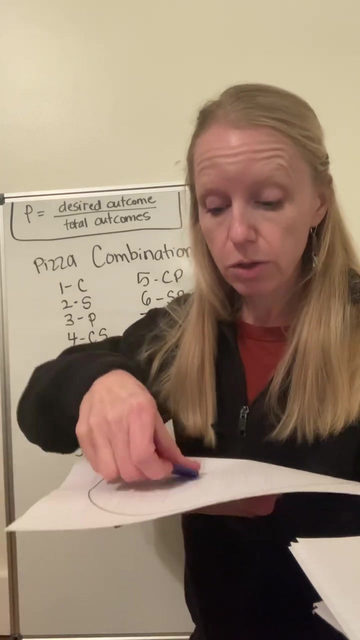 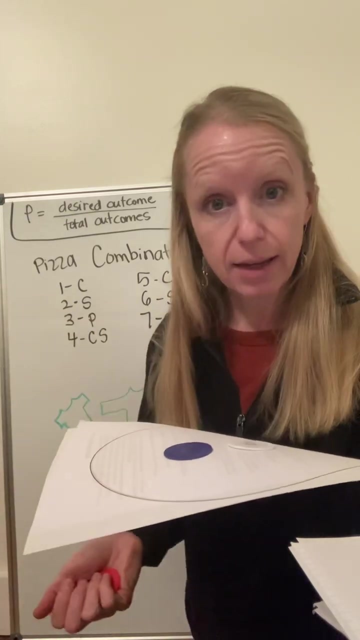 meat, whatever you want to call it, and then the whites going to symbolize cheese, and so this may help them to think through. okay, what are you going to put on your pizza? well, you could just put red peppers, or you could just put meat, or you could just put cheese, or you could put cheese and pepperoni, or cheese, and 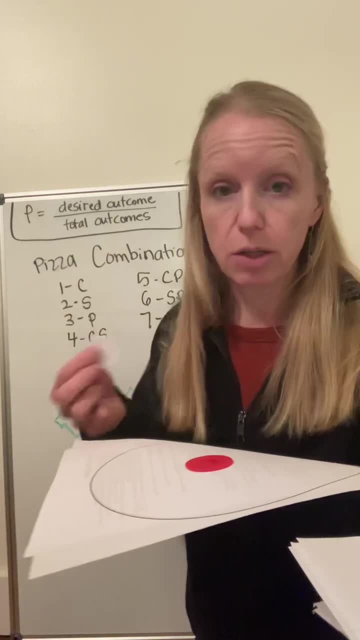 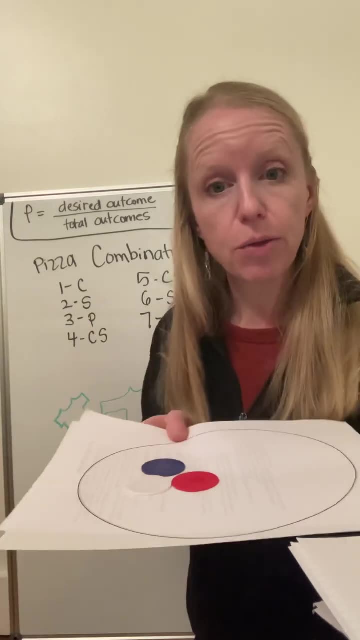 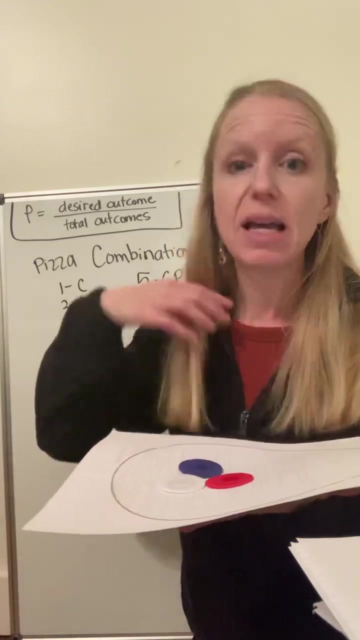 red peppers, or you could just put no cheese and just have red peppers and and pepperoni, Or you could have all three on your pizza. And so, as the kids play around and experiment with these three ingredients, I want you to write. you're going to write up here on: 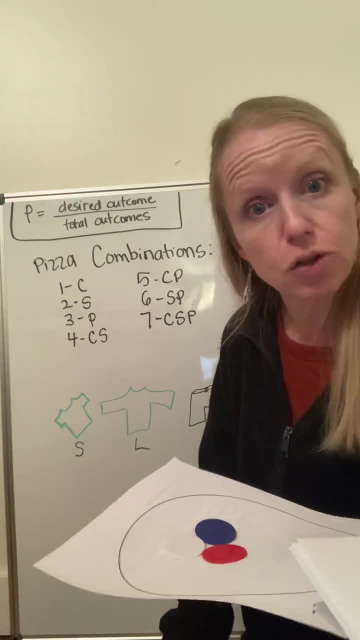 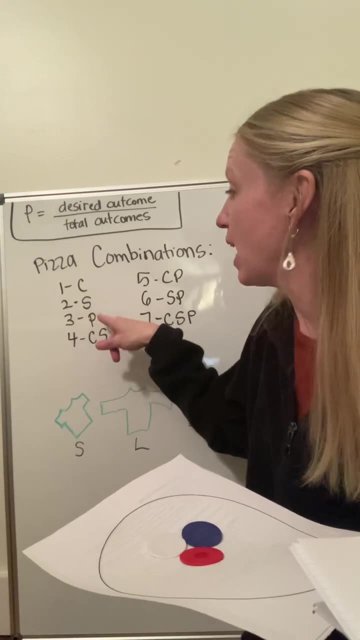 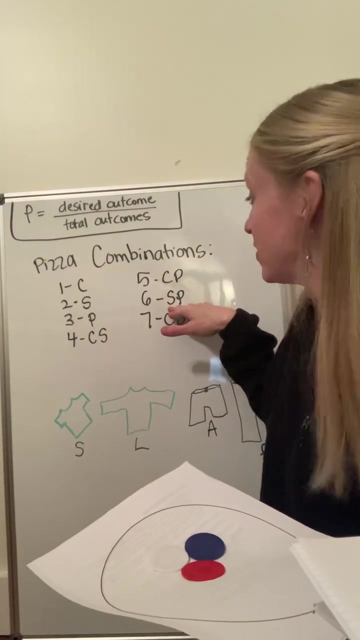 the board the different combinations of pizzas you can make. So you can make a pizza with just cheese, with just sausage- is the S I used here- or just peppers, Or you could combine cheese and sausage, cheese and peppers, or just meat, sausage and peppers, meat and veggies, Or you can have all. 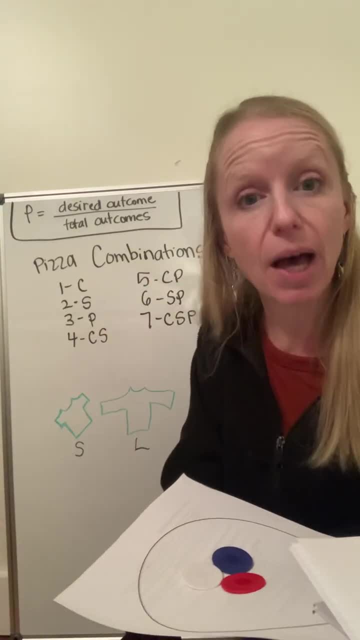 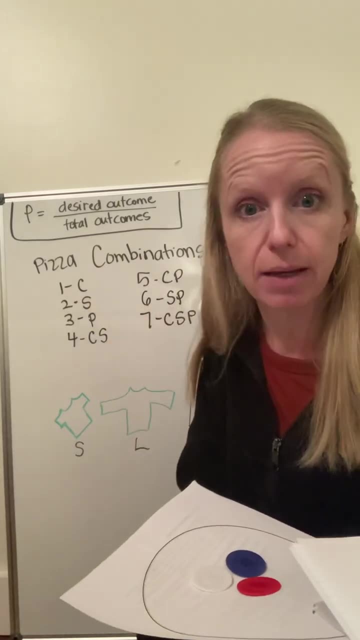 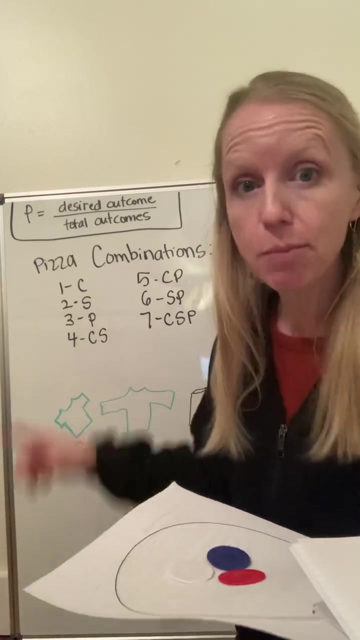 three on there, And so there are seven possible combinations. or again, arrangement of ingredients. And which pizza would you pick? And I personally would probably just do peppers. And so the chance, the probability, that I'm going to walk into the pizza place without ordering. 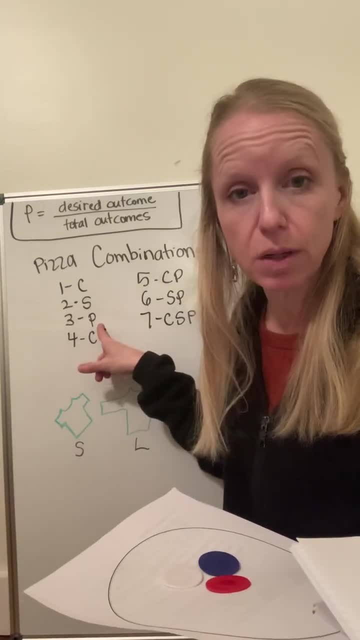 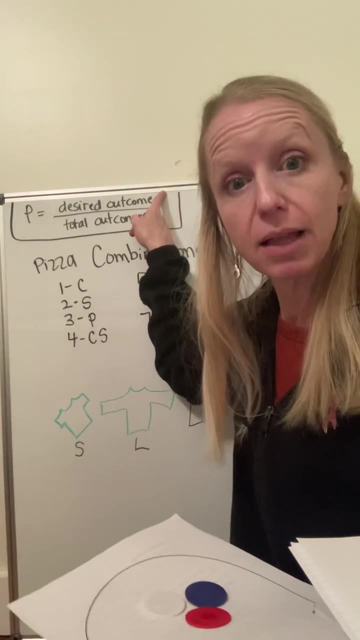 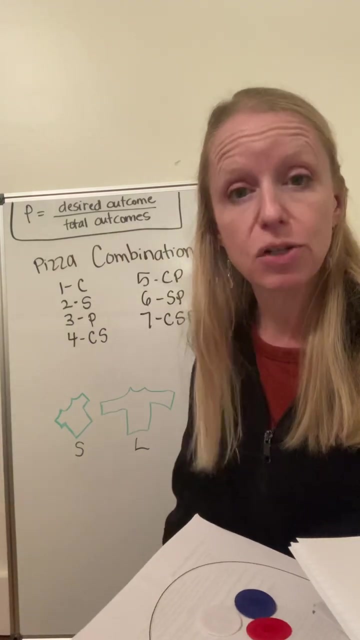 and they're going to hand me a pizza with just peppers is one out of seven. Again, probability. is your desired outcome? For me, that would be a pizza with peppers out of the total possible outcomes, which be a seven different combinations of pizza ingredients. So, again, probability. 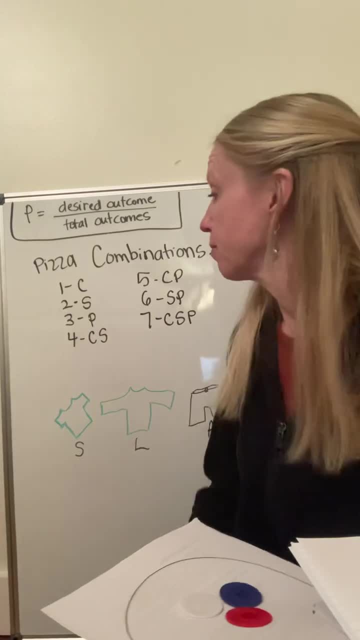 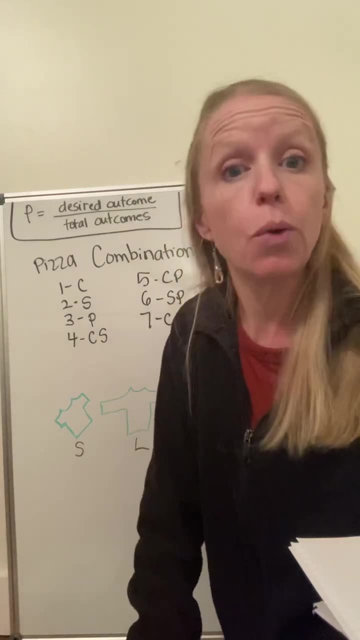 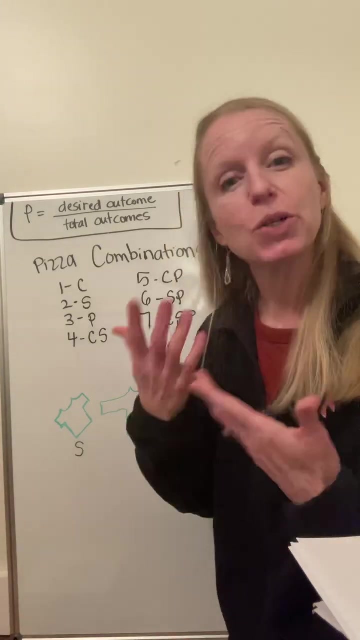 desired outcomes over your total possible outcomes. And so once you've done that and the kids have figured out, now you can't, you cannot order your pizza at this pizza place because it's a probability pizza place. And so if you were to order, then that takes away the dilemma for the most part, if they're. 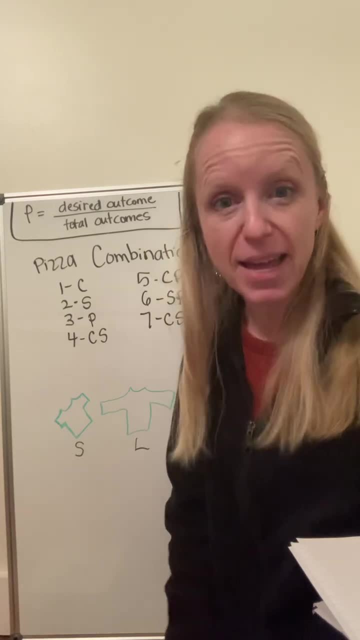 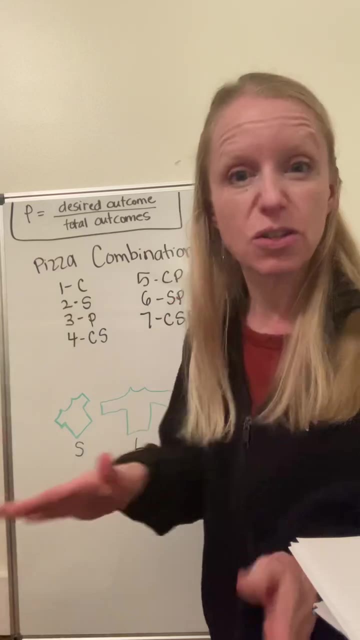 dependable pizza place, But that should at least lower your probability of not getting what you want. So this is: you don't get to order at this pizza place. That's why it's a chance that you're taking when they just hand you a pizza. So that's a possibility. And so if you were to order, then that's a chance that you're taking when they just hand you a pizza. So that's a chance that you're taking when they just hand you a pizza. So that's a chance that you're taking when they just hand you a pizza. 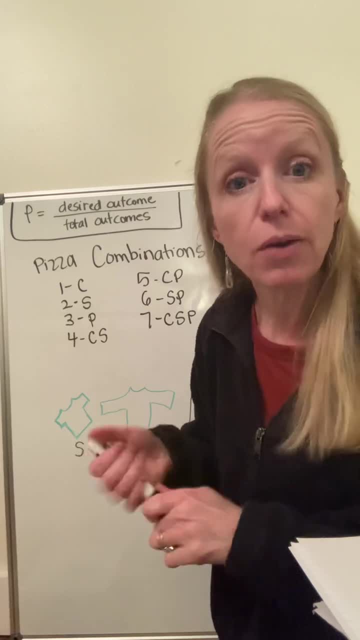 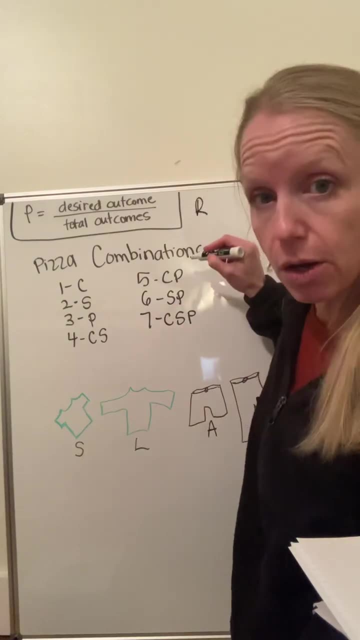 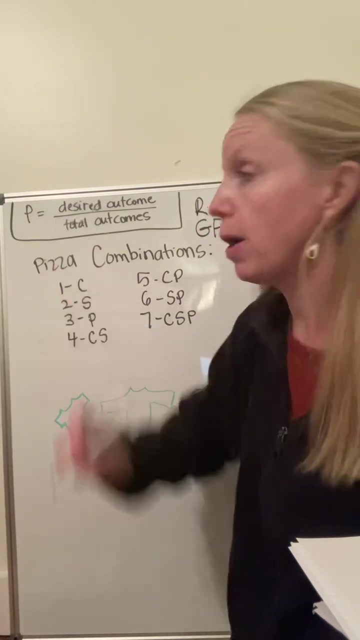 Once you've done that, you can then talk about: okay, well, what if we add in a gluten-free crust? So now you could get rather a regular crust, or you could get a gluten-free crust. So now, how many possible total outcomes do we have? So I want a pizza with peppers. 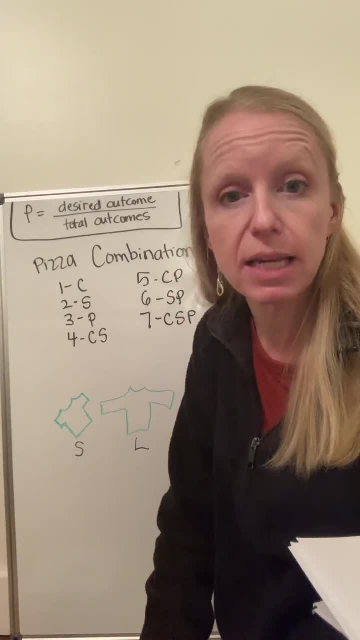 on a regular crust. So what is the probability that I'm going to get that? Well then, you're going to go back through all these things. So I'm going to go back through all these things, And so they're going to have the same ingredients, but they're rather going to have. you could put it out. 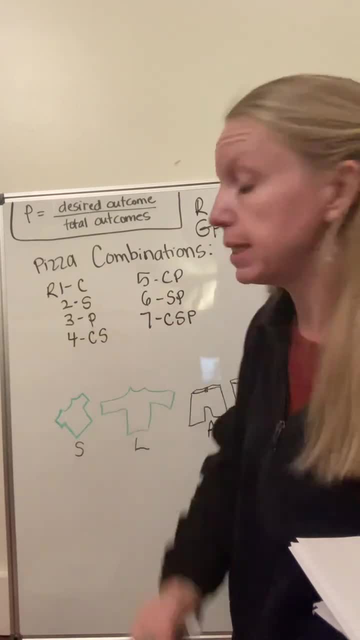 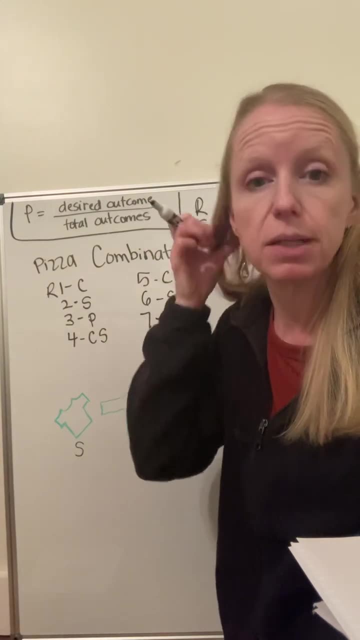 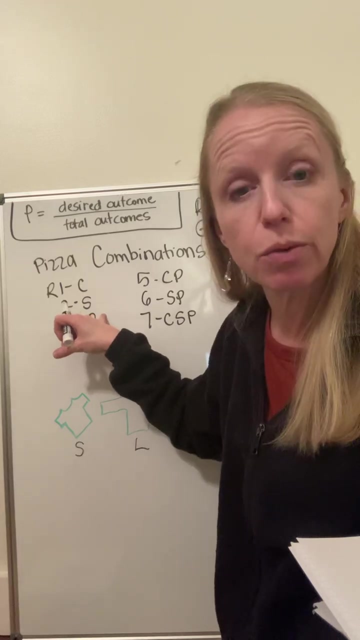 here, maybe regular crust on all of them, So that would be seven possibilities. Or they're going to have gluten-free crust on all of the same ingredients, and that would be another seven possibilities. So now we have 14 possible pizzas they could hand me, and I want the pepper with. 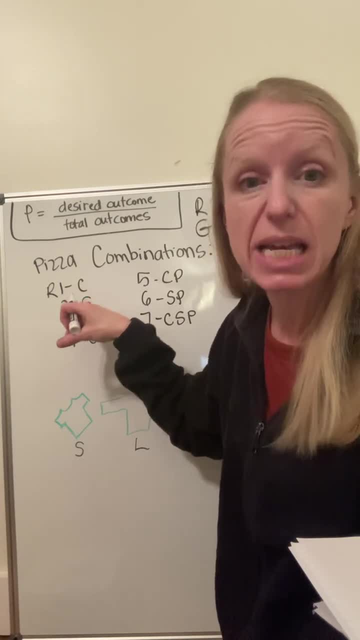 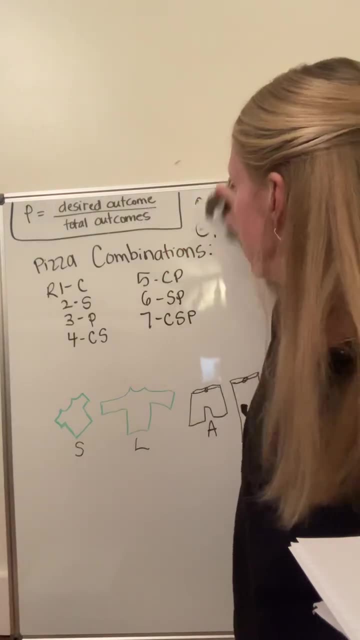 regular crust. So now my probability of getting the pizza I want is one in 14.. Again, my desired outcome over the total outcomes. Then if you want to go a step further, you could add an ingredient. So get the class to vote on what. 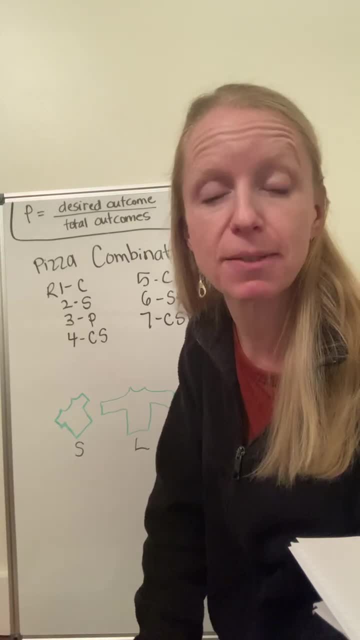 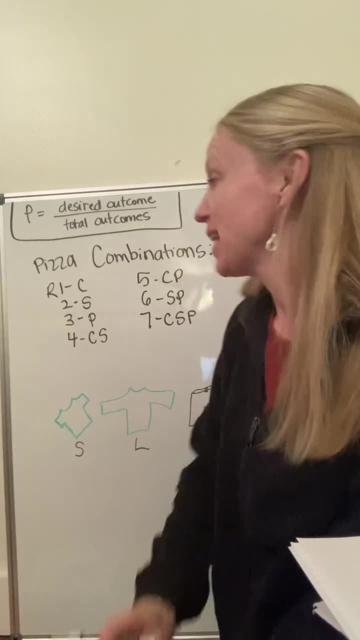 would be the other ingredient you would add to the probability pizza place And say they want to add anchovies just to be exciting. So if they added a whole other ingredient, well then you're going to go back through. They could have all these pizzas. 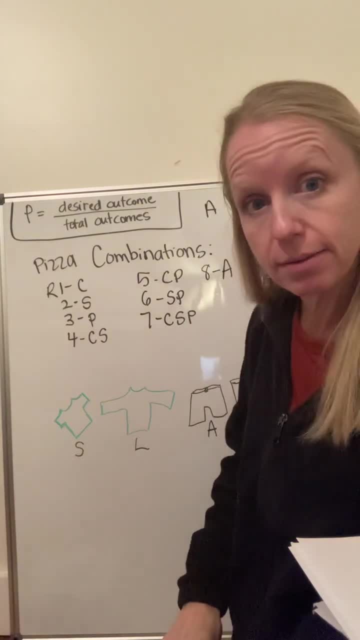 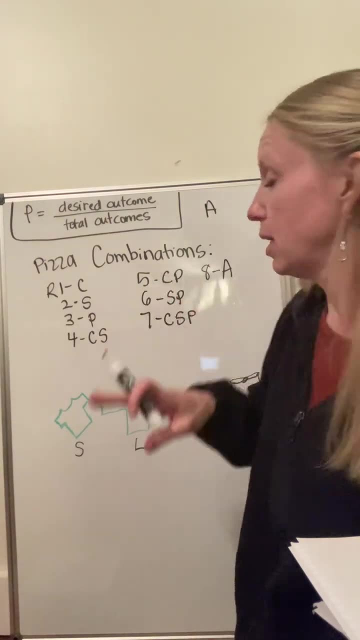 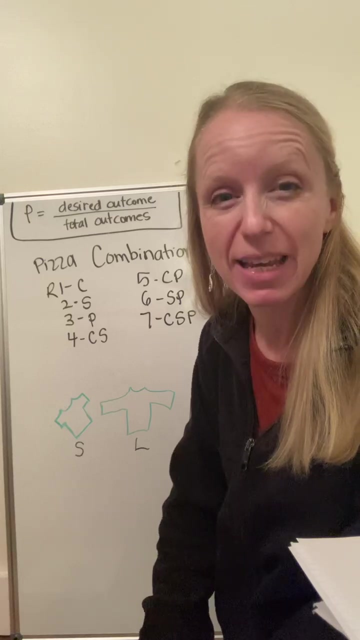 They also could have a pizza that had just anchovies, And then they could have all these different ones with added anchovies, which would be another seven, so eight different types, And so then you would end up with 15 different total possible outcomes if you just added one ingredient. 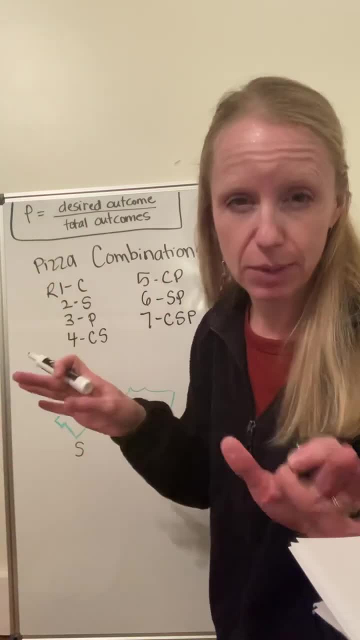 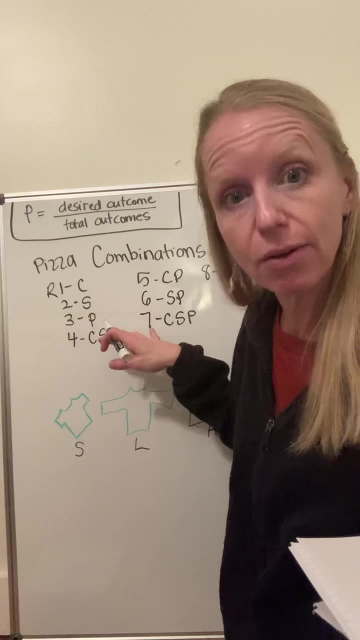 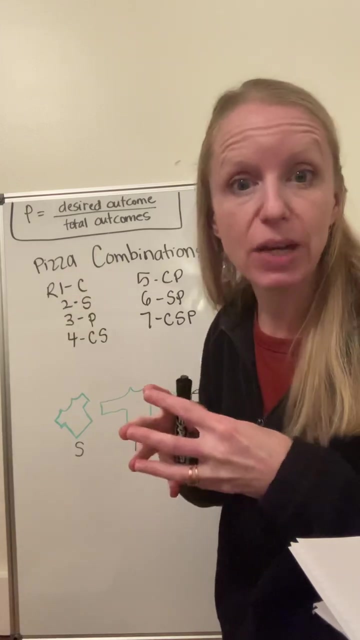 So you could continue, especially with the older kids. For the younger kids I would stop there. obviously. For the bigger kids you could add more ingredients and continue just to figure out on the board together all the different possibilities that you could have, combining different ingredients And again a combination. it doesn't matter the order that 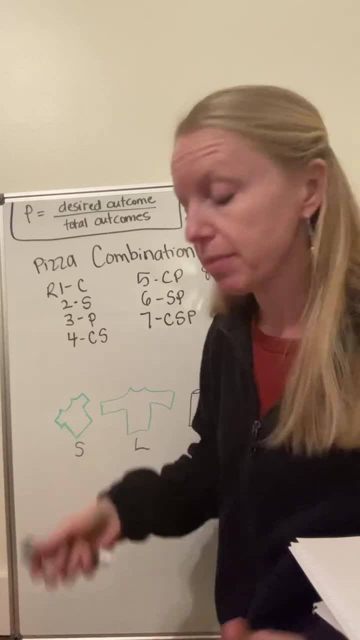 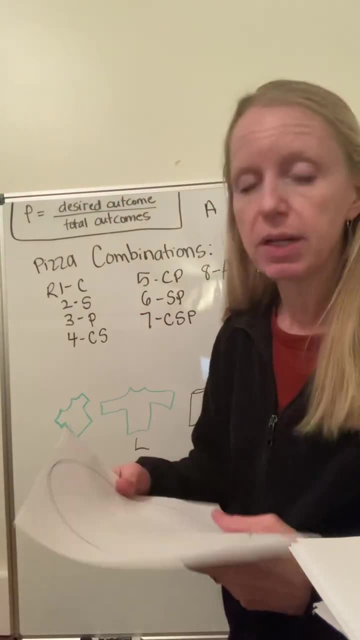 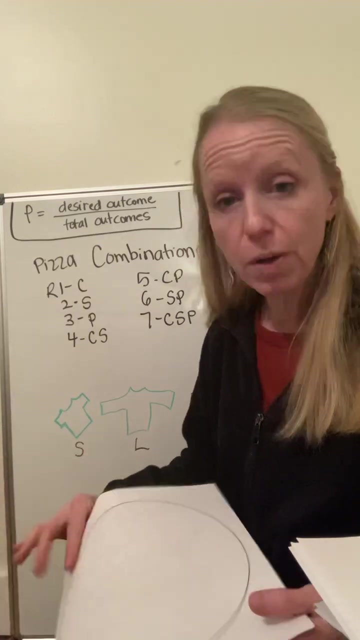 you put these ingredients in, They're all still going to be on there in whatever pizza you get And then. so then I would, you know, again, have the kids talk about their favorite ingredients. Why do they like certain pizza things, The little ones they could then, or all of them at the end? 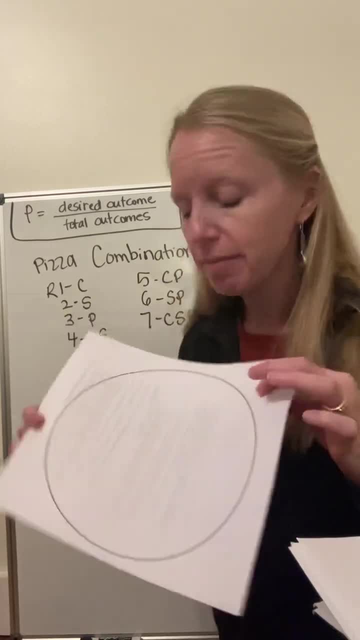 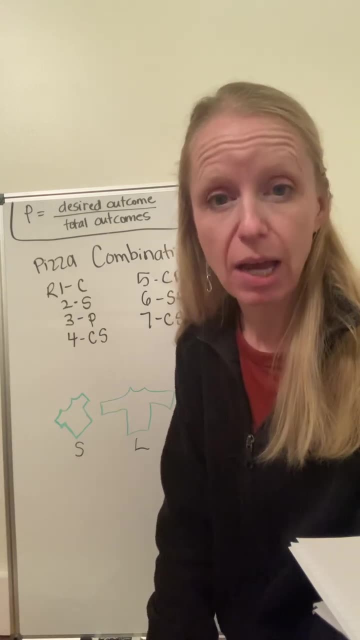 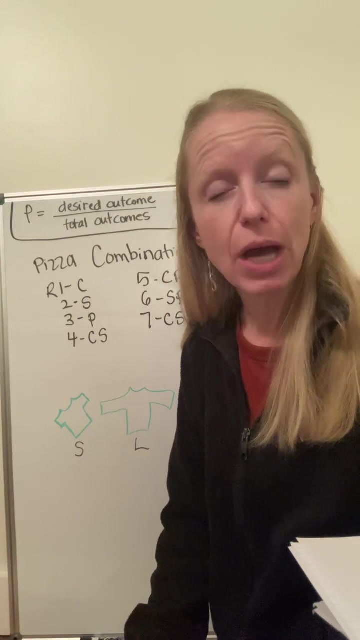 could draw their favorite pizza on their pizza crust here With their favorite ingredients and kind of go from there. Then you probably will still have some time. So then I would talk about this idea of combination probability dilemmas in our world. What are other combinations that we might? 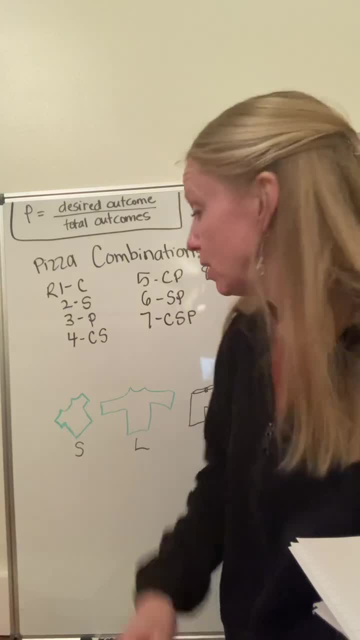 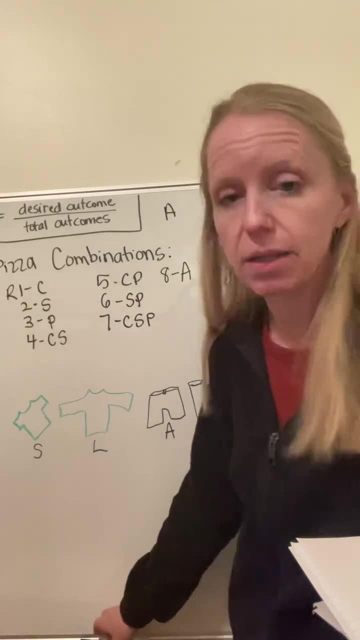 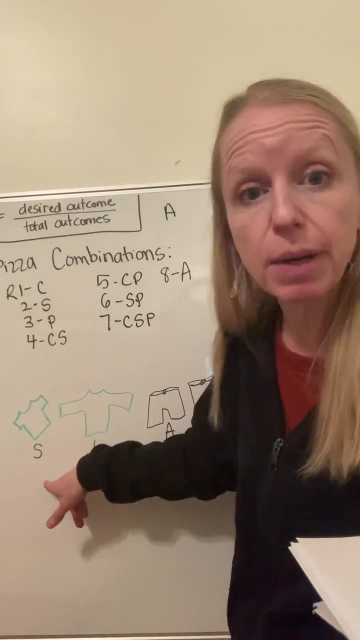 deal with on a day-to-day basis. Well, a classic one are clothes, And so I kept this one simple for our purposes. For the bigger kids you could make it more complex, But for kids just keep it simple. So say I had I needed to pick a top and a bottom to wear each day. 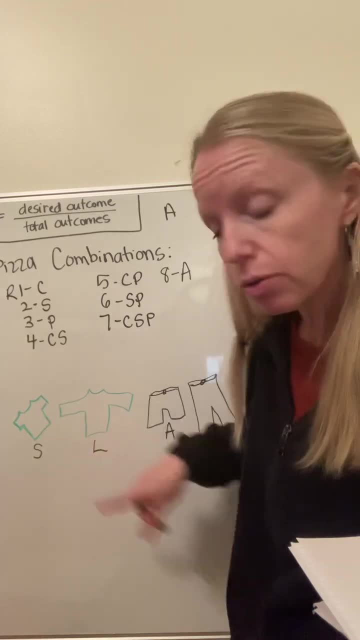 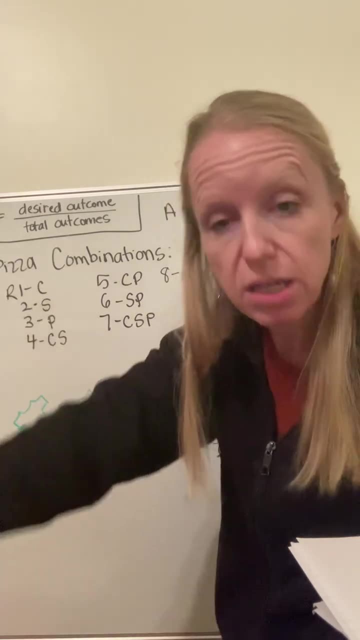 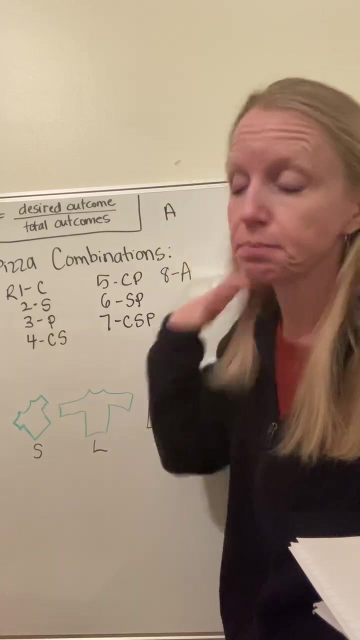 I have one short sleeve shirt, one long sleeve shirt, one pair of shorts and one pair of pants. What is the probability that I'm going to reach in and draw the shirt I need and draw the bottoms I need to fit the weather that day? Well, you know, your possible options are short sleeve. 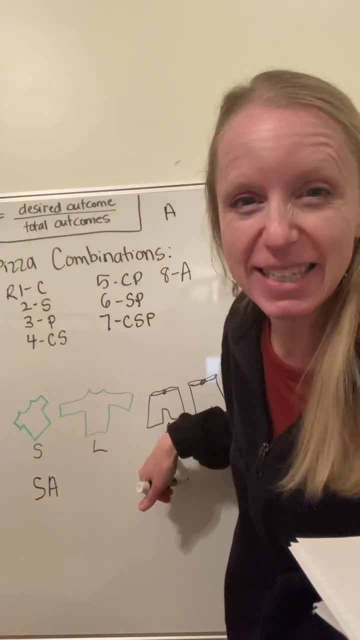 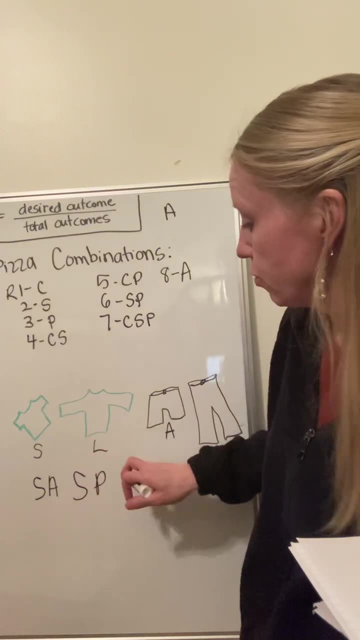 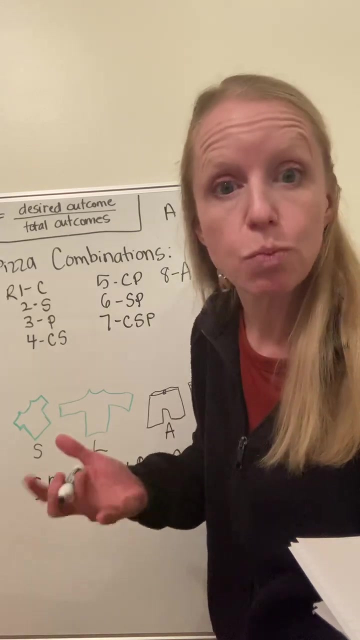 and pants and a is for athletic and it would use another s So athletic shorts, or I could get short sleeves and pants, or I could draw out the long sleeves with my athletic shorts or the long sleeves with pants. So if it was a nice warm spring day, like we had a couple of 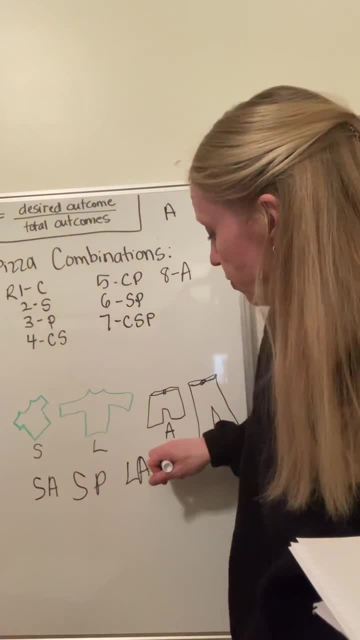 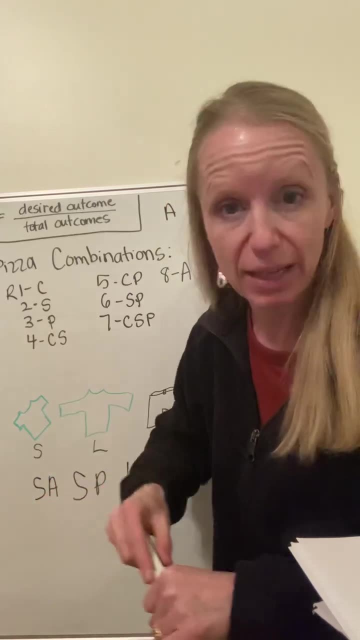 or a cold, rainy day like today. if it was a cold, rainy day today, I'm going for the long sleeves and pants And I have a one in four chance of just randomly getting that out- the probability of that. But you can do this with different colors or say you have. 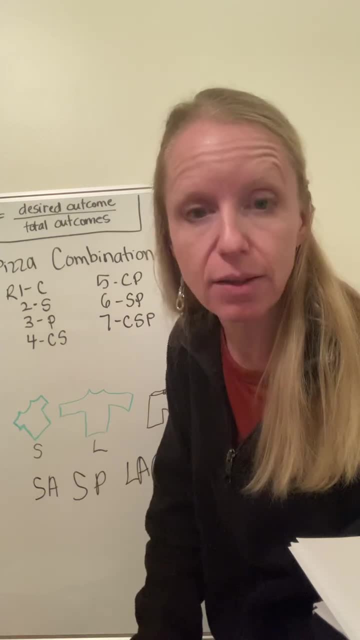 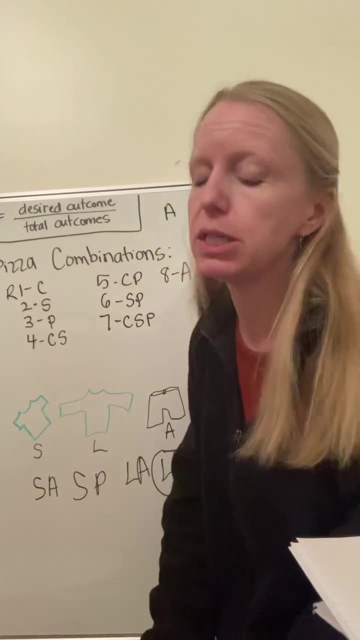 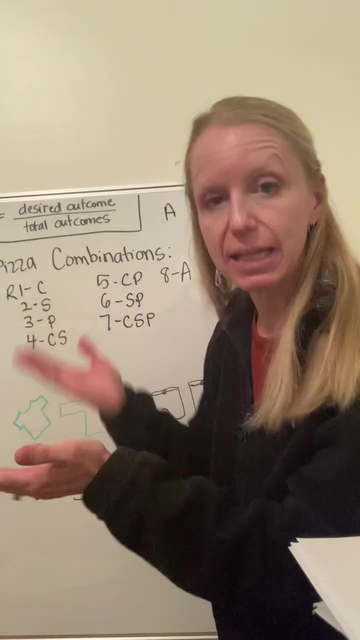 six shirts and six pants. all that are the same. How many different combinations? or you could do different color shirts and different color pants if you wanted to. How many kids could you clothe that kind of thing with just combining them randomly? So clothing is a great. 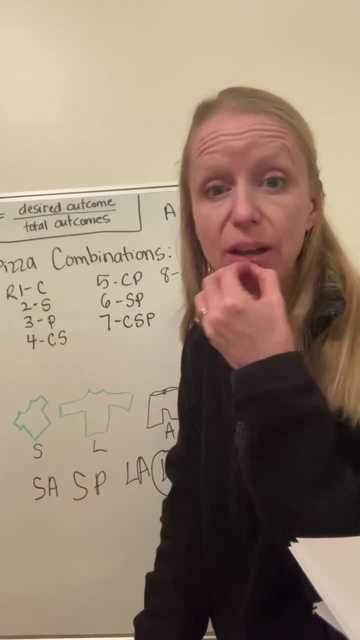 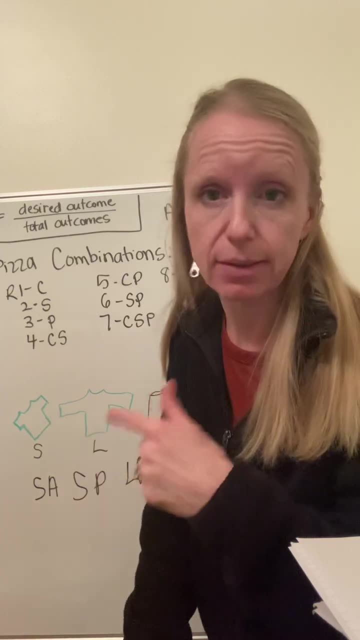 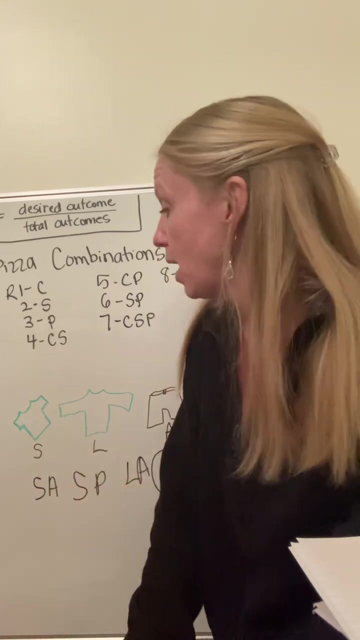 combination probability. You could also talk about cupcakes and icing or the difference. you could do different flavored icings as far as in other toppings, so sprinkles and chocolates and everything else. So you could do another food one with that Then for the older kids. so 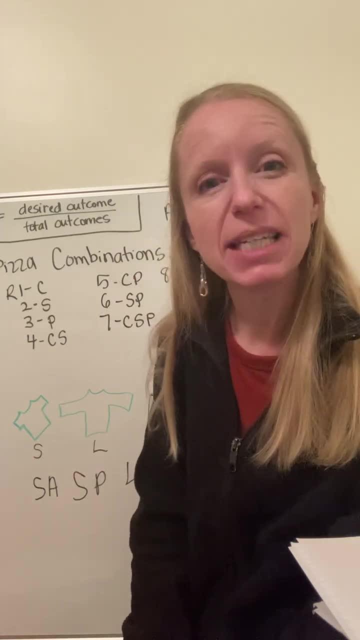 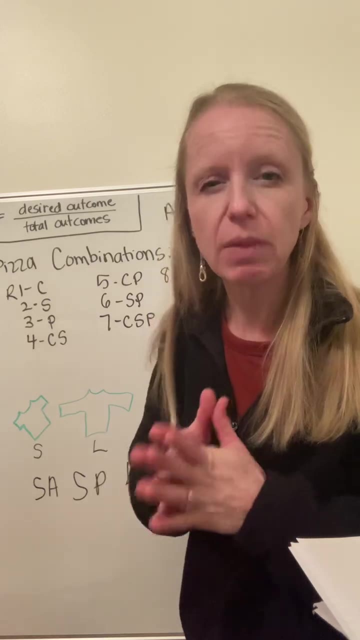 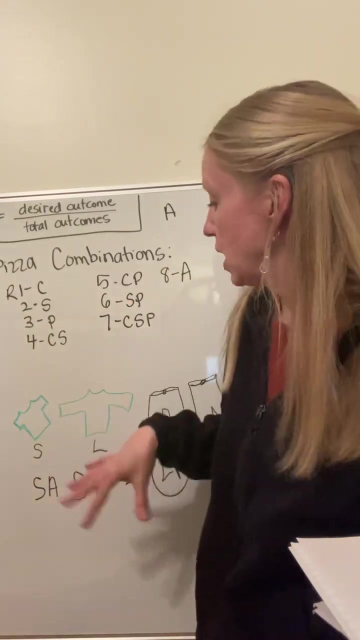 you could mention just in passing this idea of permutation. So permutation is when order does make a matter. So the classic little thing there is that combination is grouping things like we are here. we're grouping clothes. Doesn't matter what I reach in and pick out for my clothes. 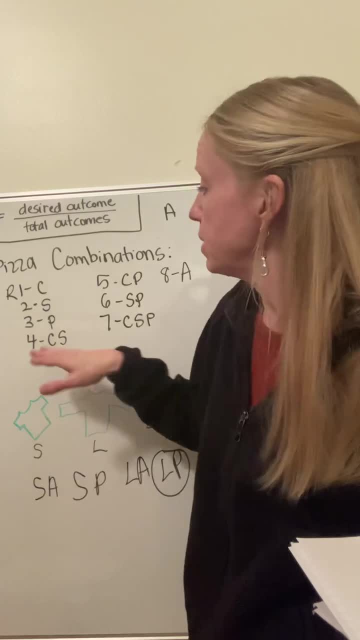 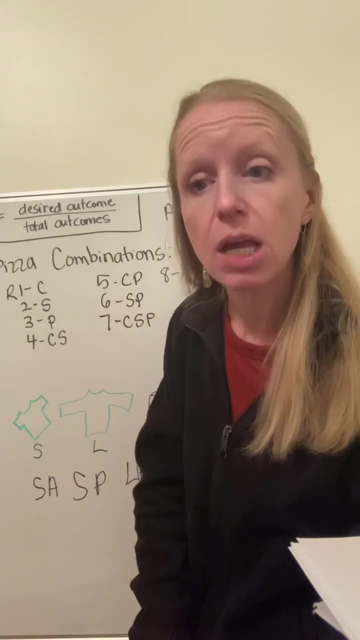 I'm still going to get a shirt and I'm still going to get some pants. Doesn't really matter what order we put the ingredients on. There's still going to be these different options, But permutation would be if you're going to list things specifically. 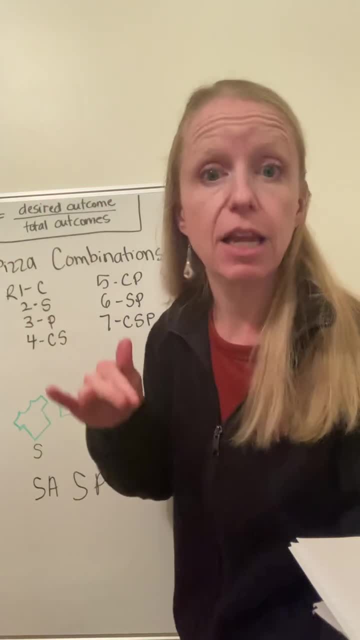 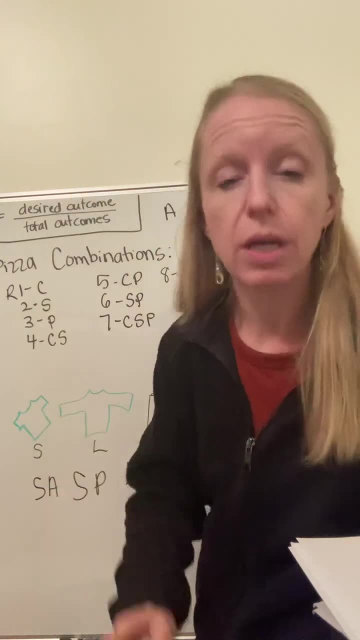 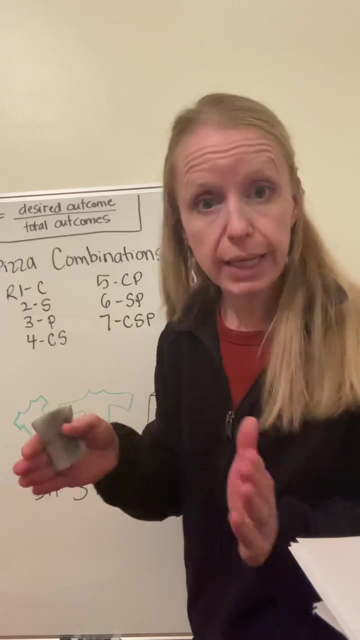 like giving places in the science fair, you're going to have a first, second, third place trophy. so if you're going to do that, the order that you do that in will change your total outcomes for each one. so if you give- say you have 20 kids- you give one first place. then your options, your 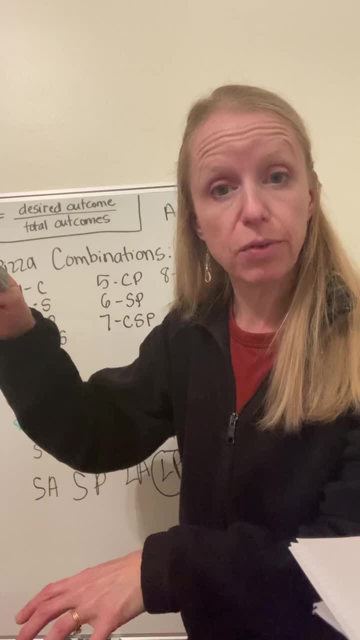 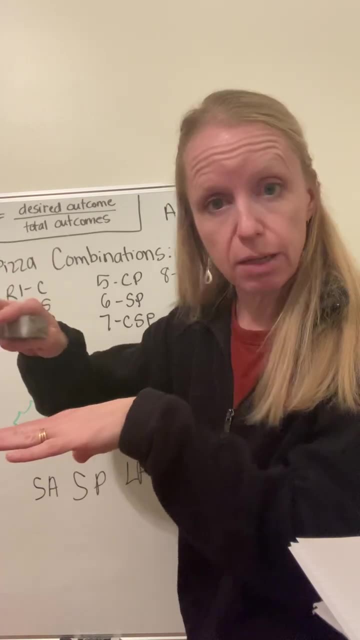 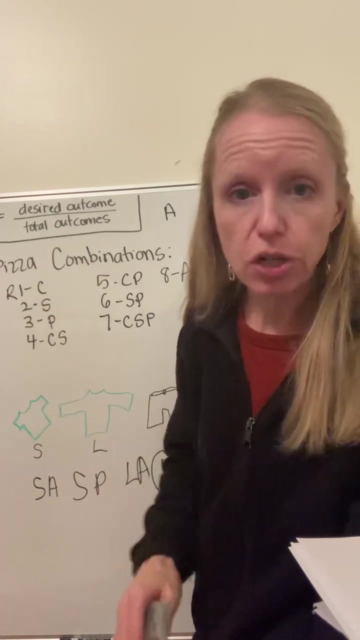 total probability for how many total outcomes could be for second place is going to be 19 instead of 20.. your third place- now you already have a first and second place. your third place- your total outcomes, is going to be 1 out of 18.. and so it's going to change your actual total outcomes and